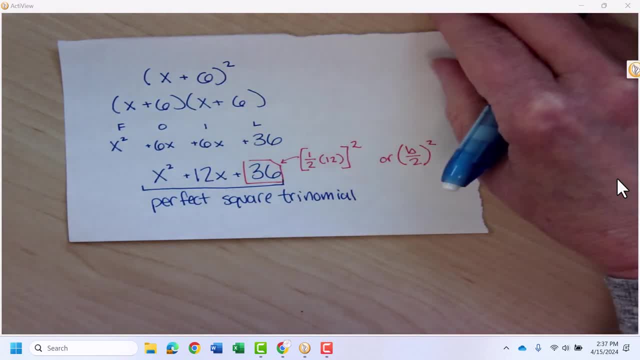 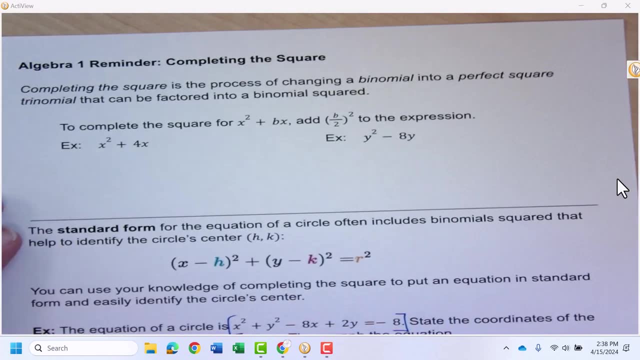 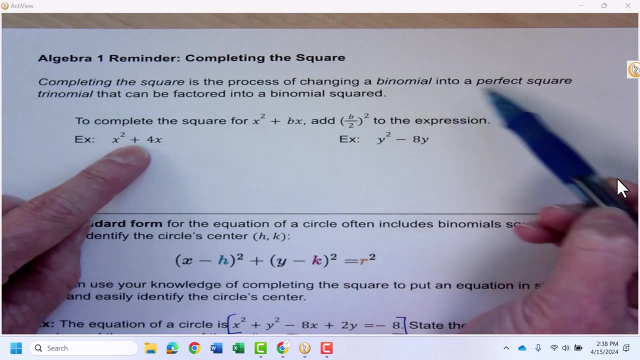 And if you already know how to complete the square, you can just go ahead and fast forward onto how to tackle the problem at hand At the top of the notes that I'm continuing on here. completing the square is the process of changing a binomial like this one into a perfect square trinomial. 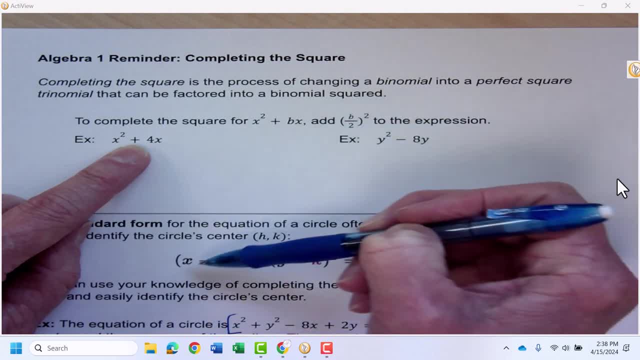 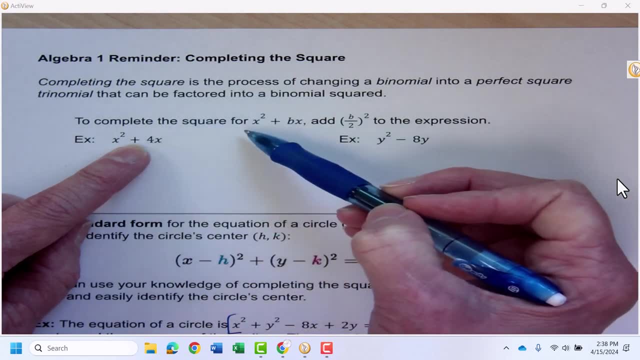 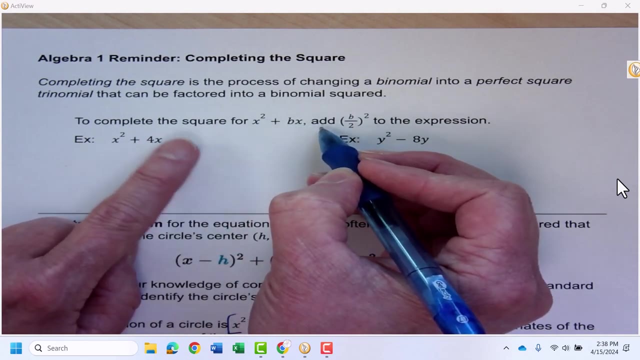 so that it can be factored into a binomial squared, like the things that we'll need in standard form for the equation of a circle. To complete the square, if I have an x squared term and an x term, I just need to add on one more term. And that one more term that I'm adding on. 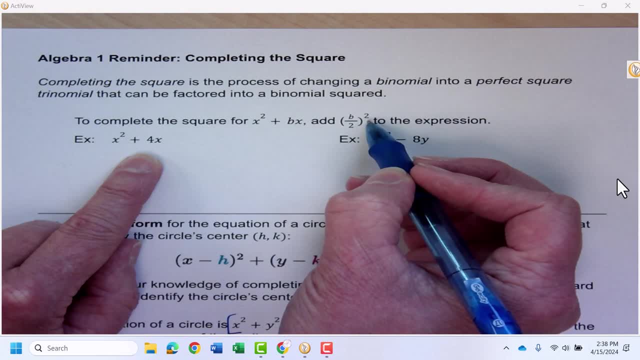 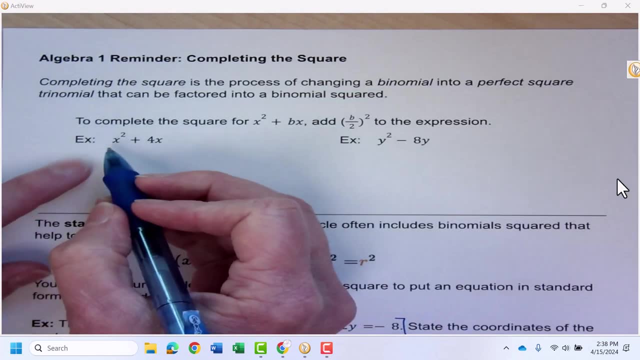 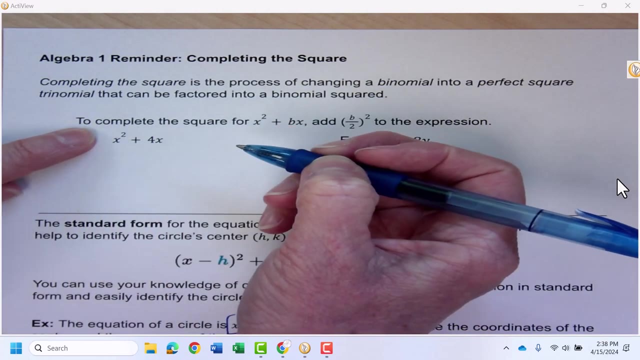 is half of whatever b is squared. So let's do it a couple of times, just so we can see how that's done, and then we'll use it. So here I have a binomial. The leading coefficient is 1.. And if I want to create a perfect square trinomial, I'm going to take 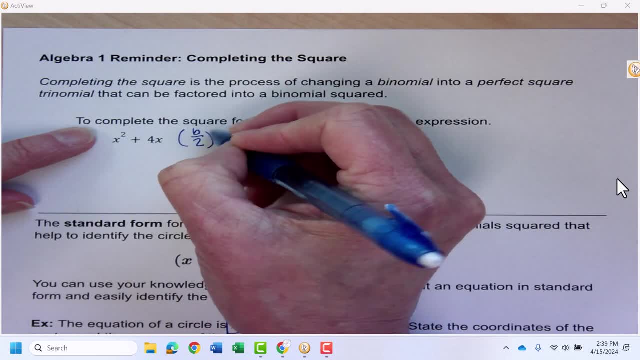 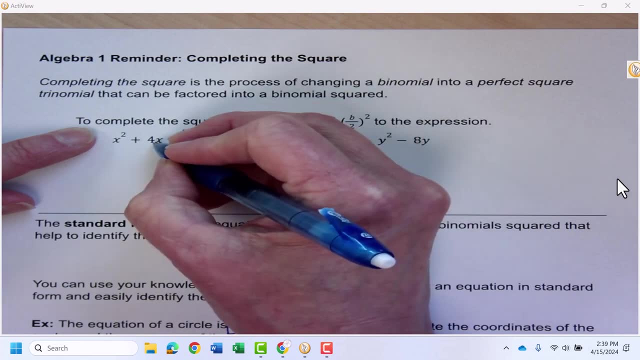 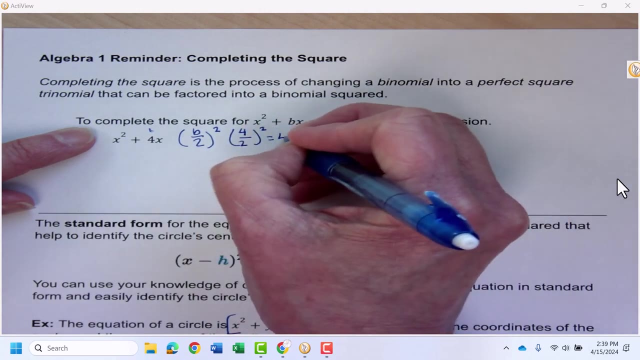 the number in front of x, split it in half and square it, So in this case that's going to wind up being 4. That's the value of b divided by 2 squared. So 2 squared That's the number I need to add on to this in order to have a perfect square. 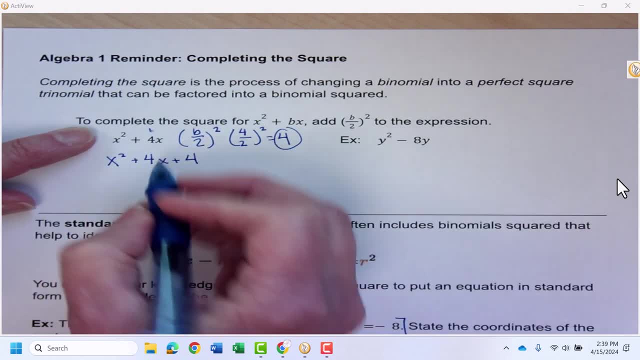 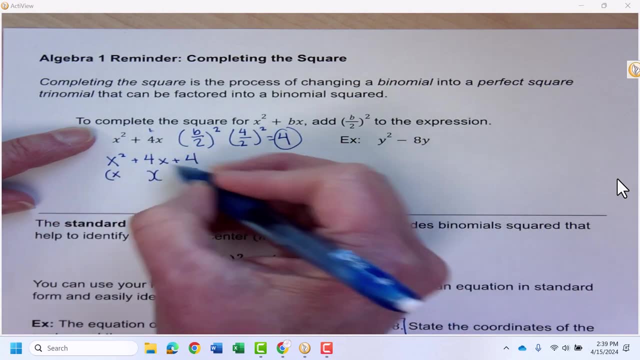 trinomial And, to remind you, a perfect square trinomial can factor into a binomial squared. Two numbers that multiply together to give me 4 and add together to give me 4 are 2 and 2.. x plus 2 times x plus 2 can be: 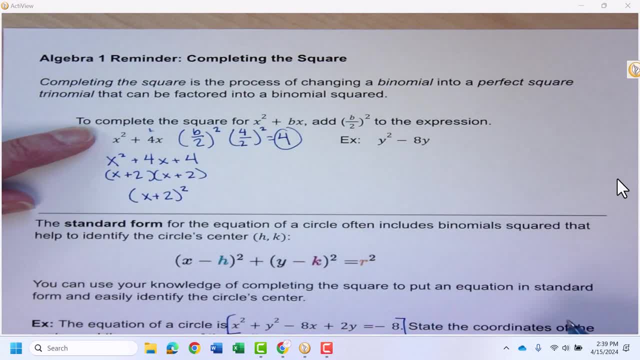 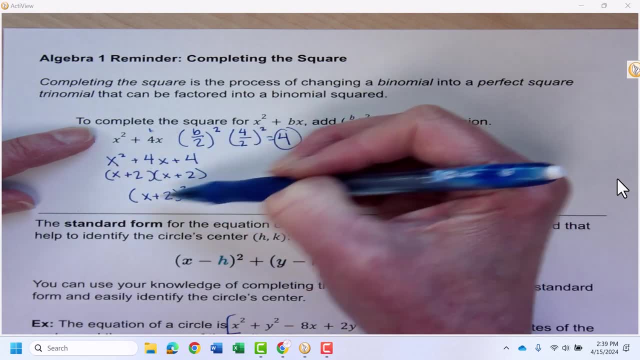 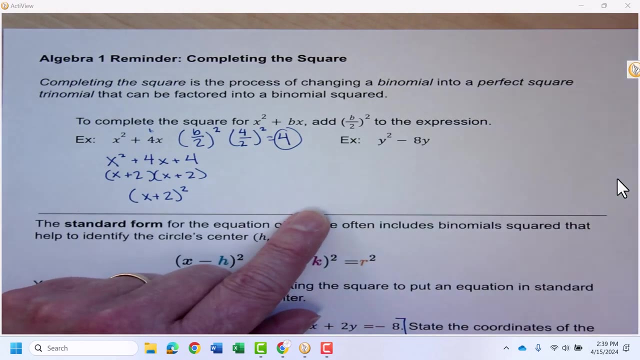 expressed as x plus 2 squared. So by taking half of 4 and squaring it and making a perfect square trinomial, I can create a binomial squared like what we'll need in our standard form down here. Let's do it one more time. I'll do it in a different color. 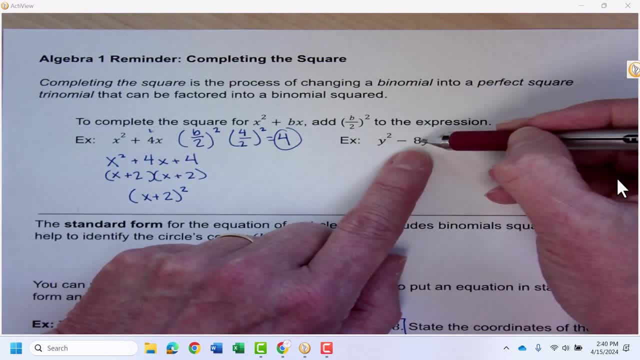 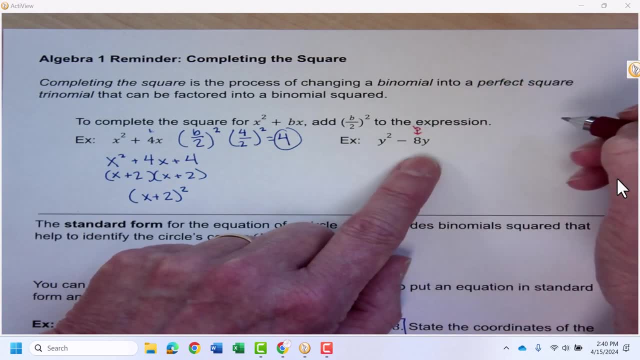 So one more time I have a squared term and just the variable term here. In this case the value of b is negative, Negative 8, I'm going to take half of b and square it. So half of negative 8 is negative 4, and negative 4 times negative 4 is positive 16.. 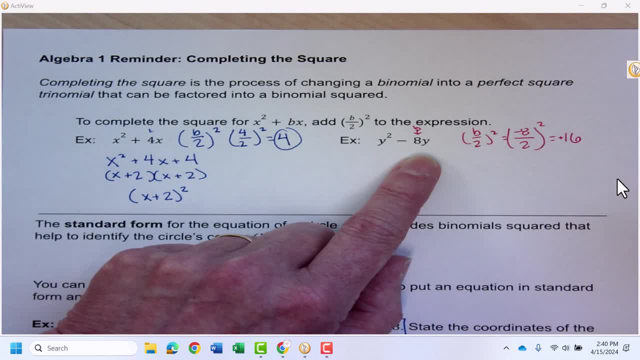 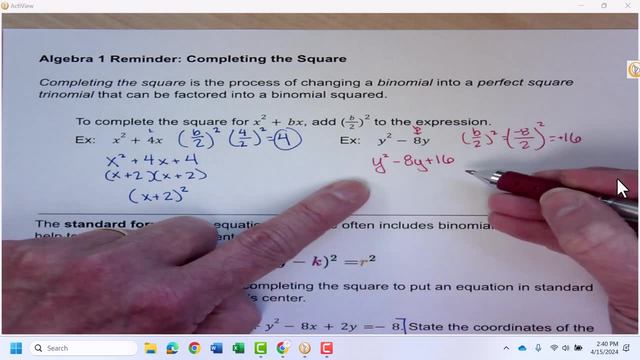 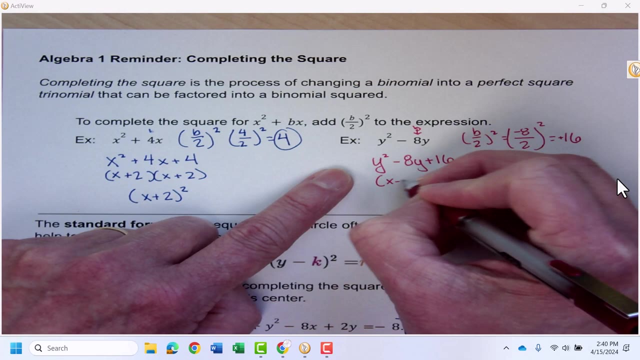 Because I'm squaring it, that number that I'm adding on is always going to be positive. So to complete the square, There it is, And the two numbers that multiply together to give me 4, and add together to give me negative 8, are negative 4 and negative 4.. 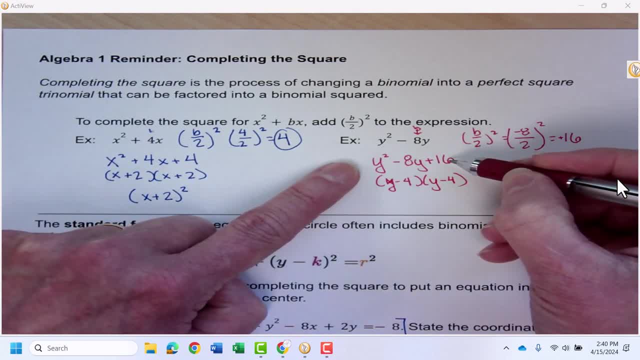 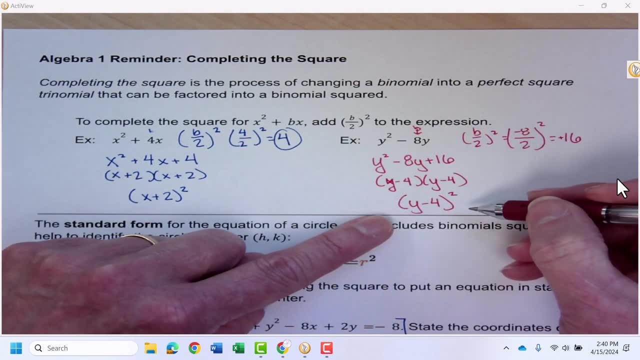 If I multiplied this out, I'd have this perfect square trinomial, and because it's the same thing multiplied by itself, I can express it as a binomial squared. Okay, so now that we know how to complete the square, so we have a binomial squared. 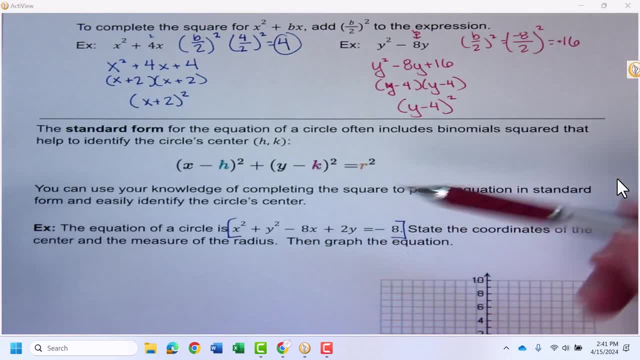 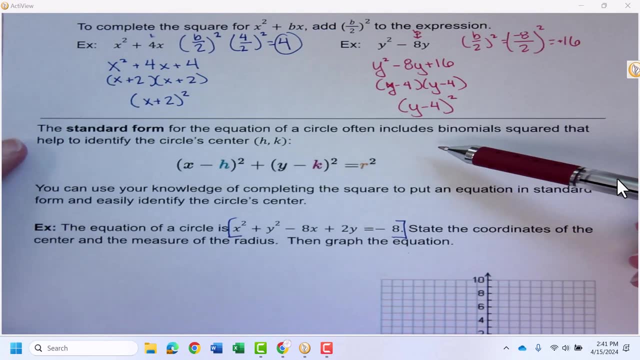 let's go ahead and apply that to this last problem. You'll have one of these in the practice assignment tonight. So the standard form of the equation of a circle has binomials squared, and those are the things that help us to identify the center of the circle. 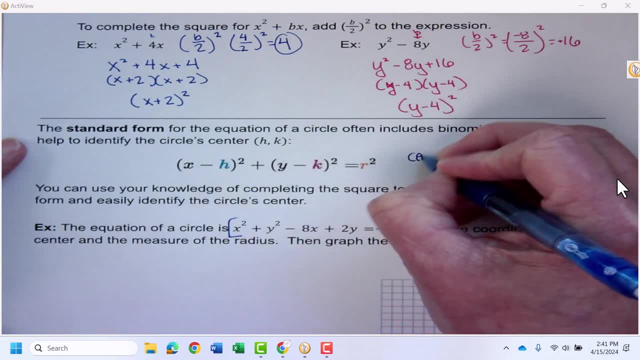 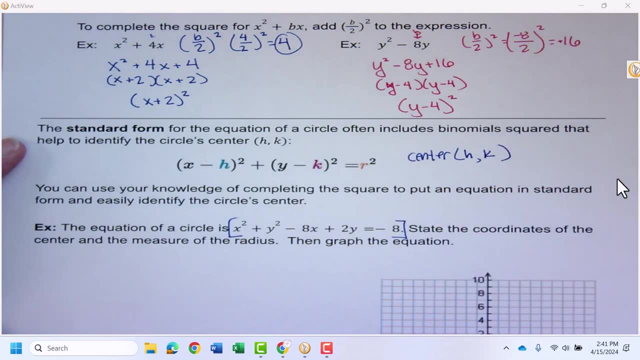 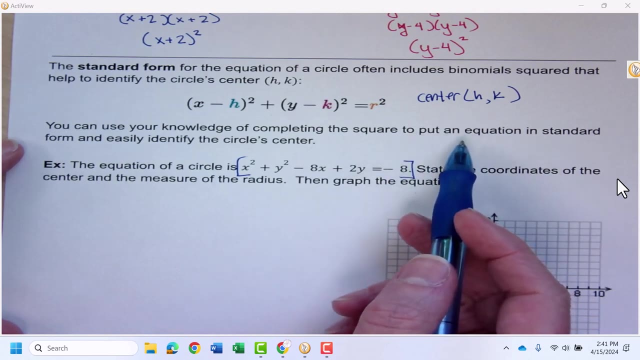 In this formula the circle's center is the value of h for the x value and the value of k for the y value of that center. So we can use our knowledge- We have the knowledge of completing the square- to put an equation in standard form and easily identify that circle's center. 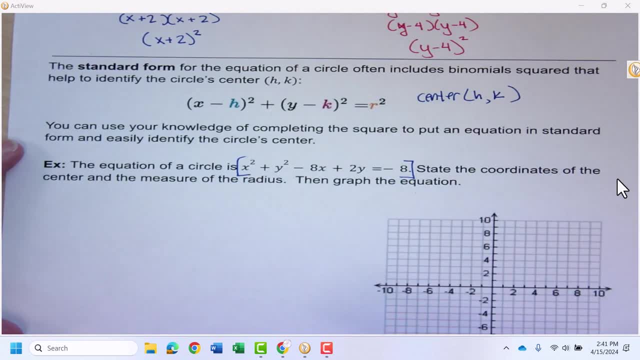 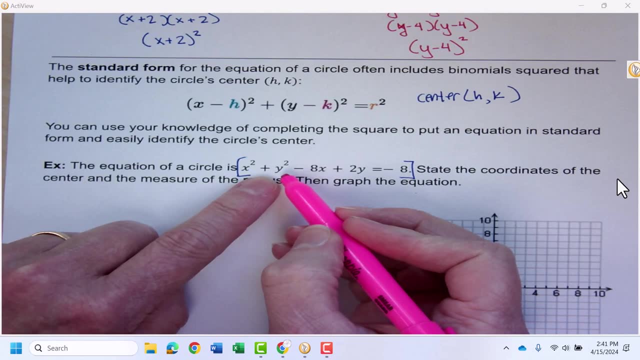 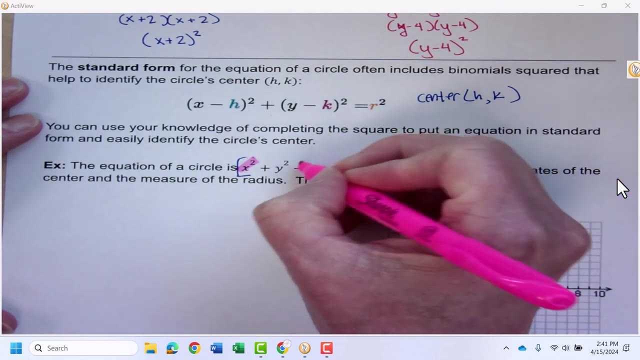 So this is not in standard form, but we can put it there. Watch how we can do this. So I have x squared plus y squared minus 8x plus 2y equals negative 8.. Well, I'm going to pull together all the things that have x in them. 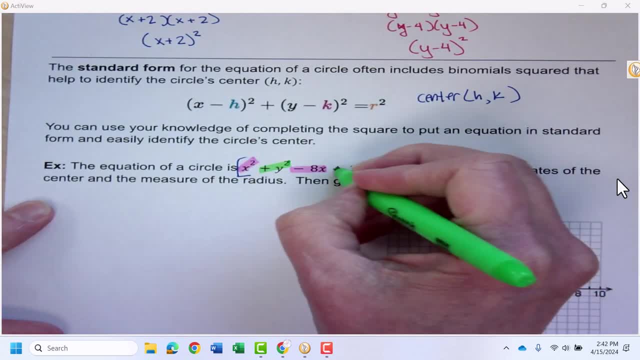 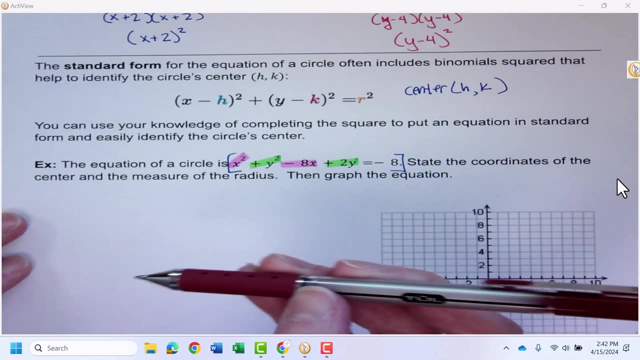 and I'm going to pull. I'm going to pull together all the things that have y in them and I'm going to create a binomial squared. So I'll keep the color coding going here. I have x squared minus 8x. 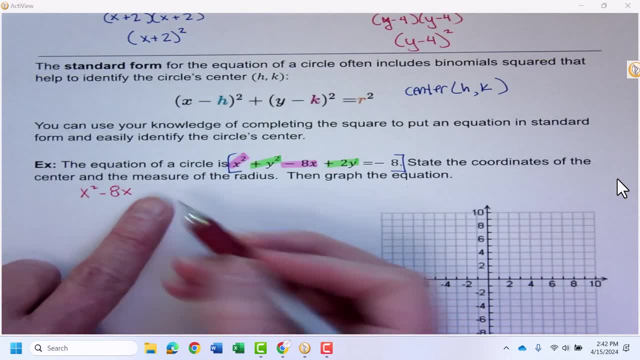 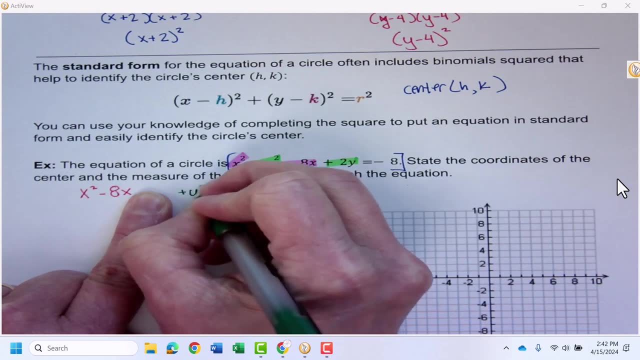 Now, I'm going to complete that square in just a moment, so I'm going to leave a little bit of space here. And I have y squared plus 2y And again I'm going to complete this, So I'm going to leave a little space. 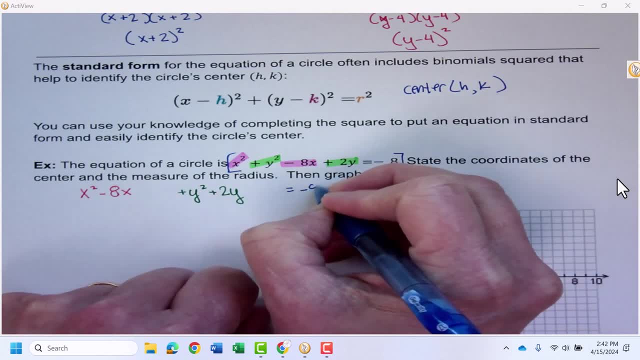 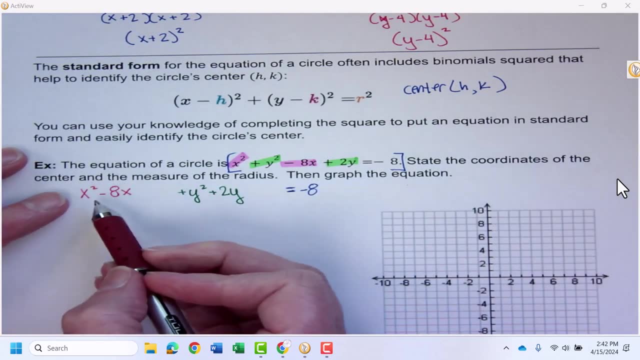 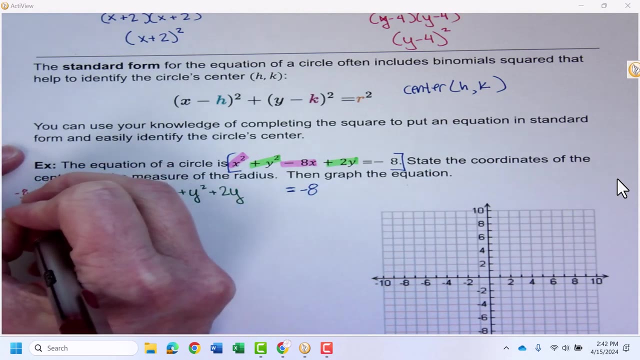 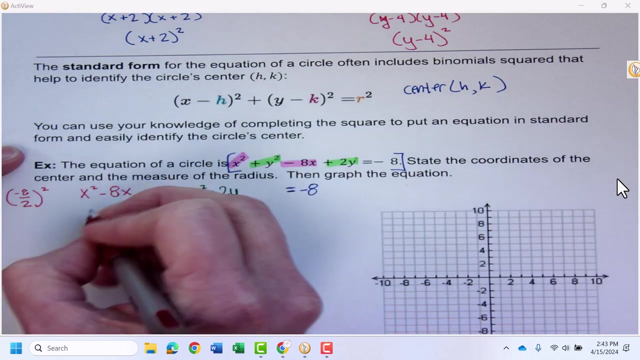 And that's going to be equal to negative 8.. Let's go ahead and do this. keeping in mind that this is an equation, Let's complete the square here. I'm going to take half of negative 8 and square it. Negative 4 squared is positive 16.. 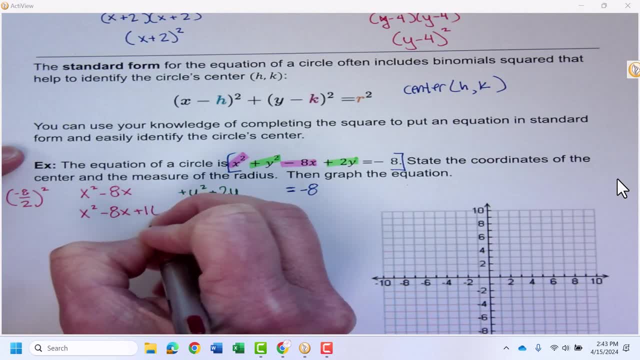 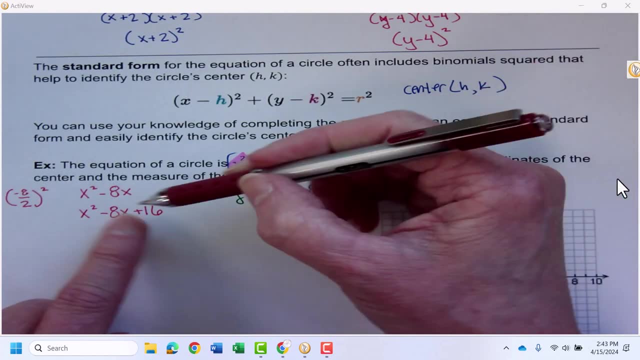 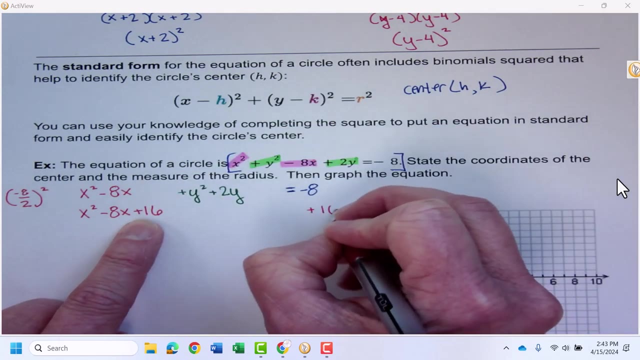 Now let's remember that I'm not just completing the square. I'm in the middle of an equation here And I just added 16 to the left side of this equation. So I better add 16 to the right side of this equation. 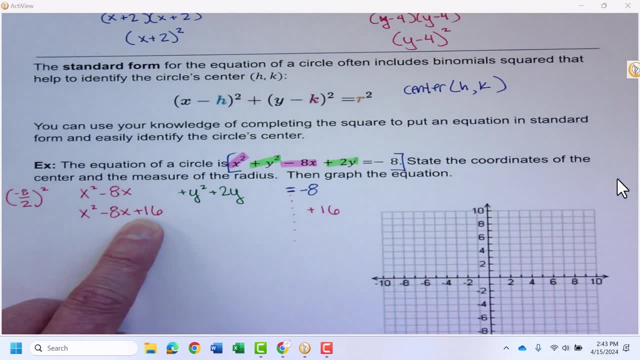 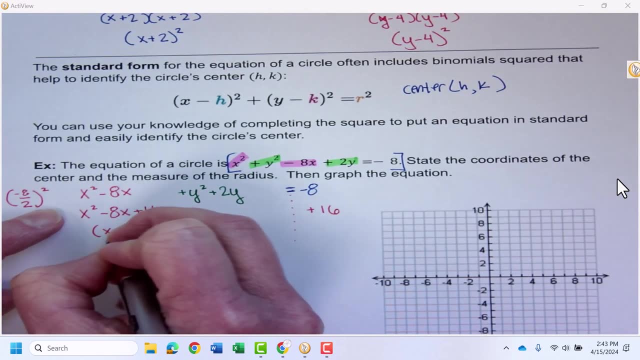 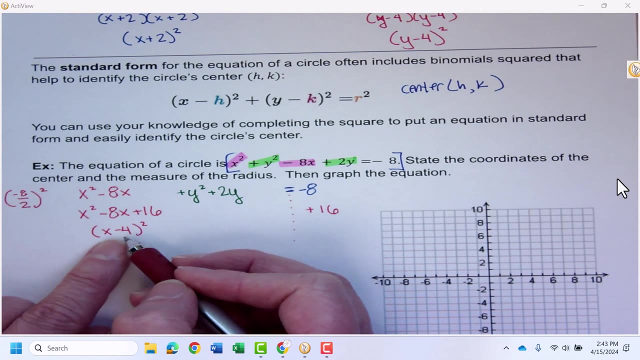 so that I keep the equation balanced, Let me go ahead and change this from a perfect square trinomial to a binomial squared. Negative 4 times negative 4 would be positive 16.. And negative 4 plus negative 4 would be negative 8.. 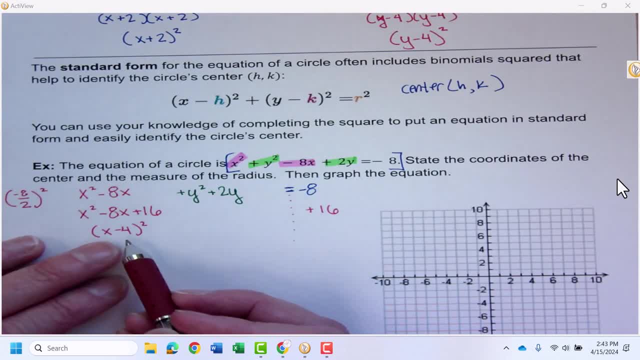 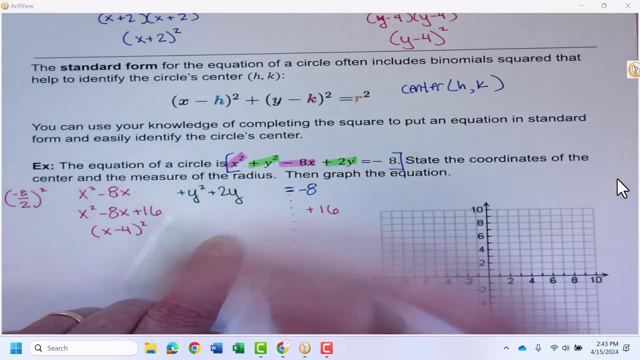 All right. so now I know the x value of the center of my circle. Let's go through this same process to find the y value for the center of my circle. All right, one more time. I'm just going to do it on this paper here. 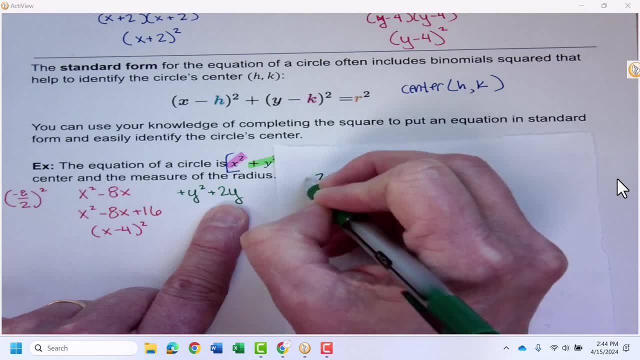 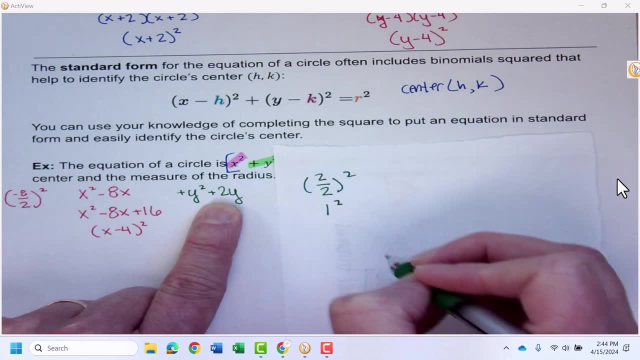 I'm going to take half of b and square it. This is the b value: 2 divided by 2 is 1 squared And 1 squared is just 1.. So I'm just going to be adding on 1 to complete the square. 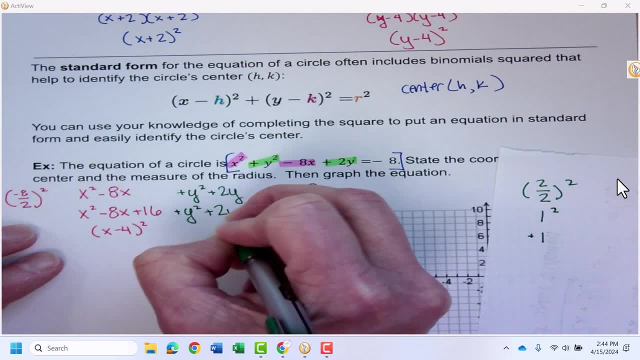 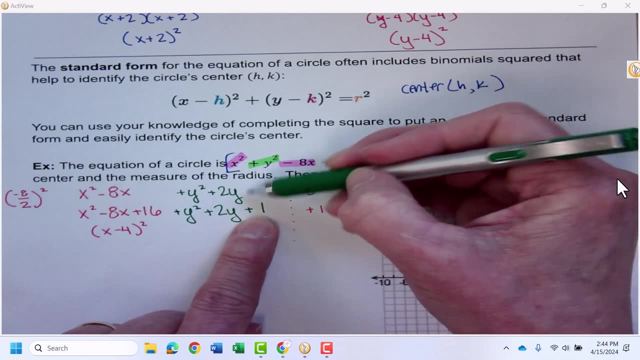 So here is y squared plus 2y, And I'm adding on 1 to complete the square. Now, just like I did before, I added 1 to the left side of the equation, so I better add it to the right side of the equation as well. 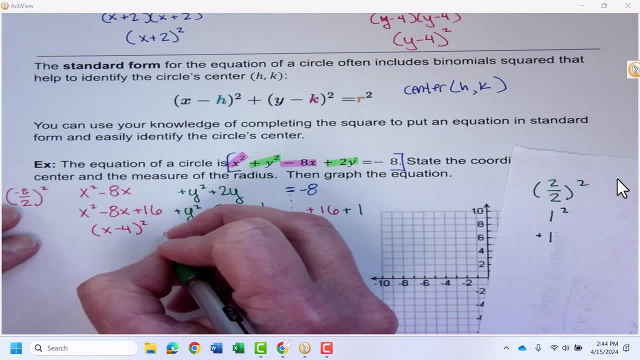 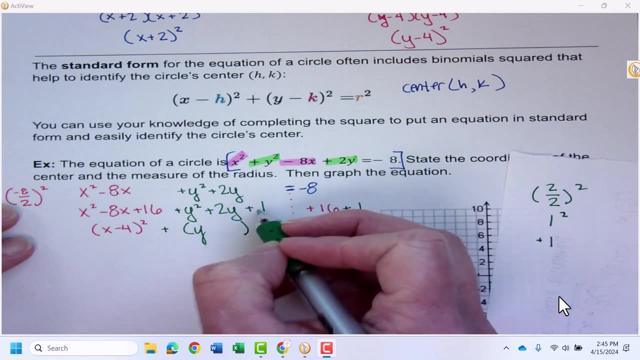 And now I can write this. And I can write this as a binomial squared. Sorry, there was just a little interruption there. Two numbers that multiply together to give me 1 and add together to give me 2.. 1 and 1, so that's y plus 1 squared. 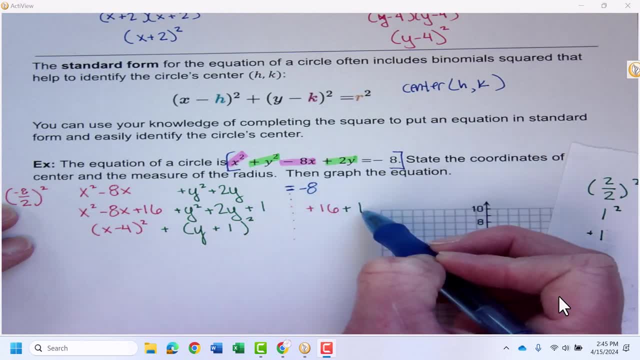 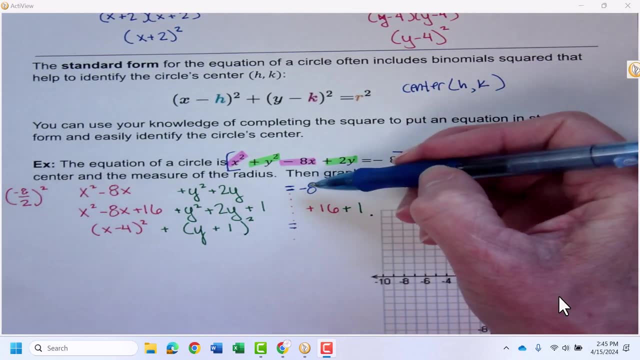 All right. when I added the 1 to the left side of the equation, I added it to the right side. When I added 16 to the left side, I added it to the right side. Over on this side, I started with negative 8..